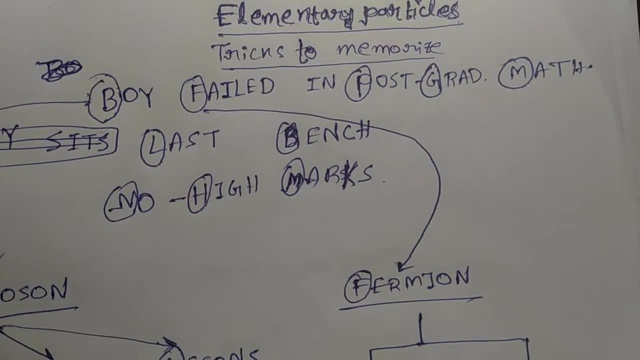 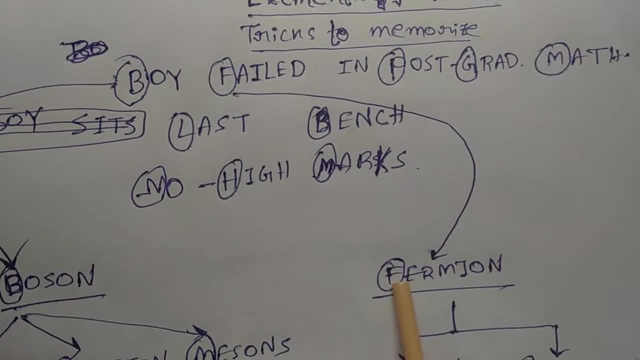 Hello friends, today we are now going to discuss how to memorize elementary particle table list. Now let's start. We know that there are two types of particle. One is boson, another is fermion. There are two types of particle- elementary particles- And how to memorize this two. 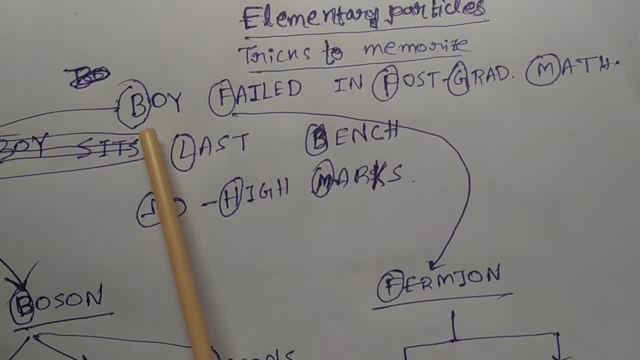 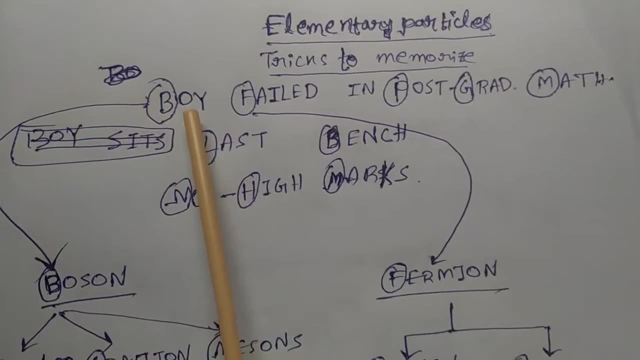 the name of the two types of particle. You have to memorize this line: Boy failed in post-grad math. Boy failed in post-graduation math. Okay, boy B for boson F, F for fermions And post-grad math. 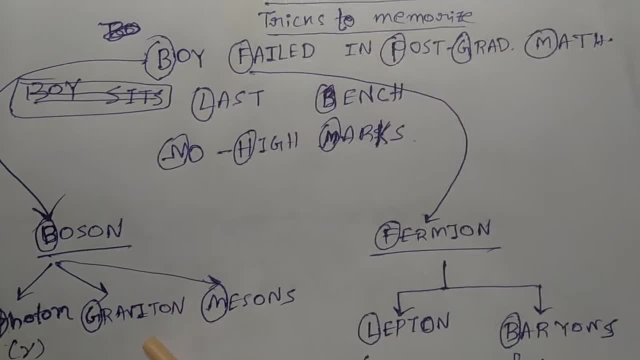 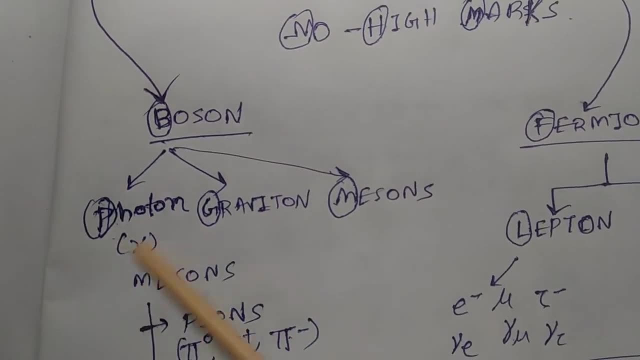 P for photons, G for graviton, M for mesons- Photon graviton and mesons. there are three types of classification of bosons And what are the classification of photons? There are no types of classification of photons. there are no classification of gravitons, but there are three. 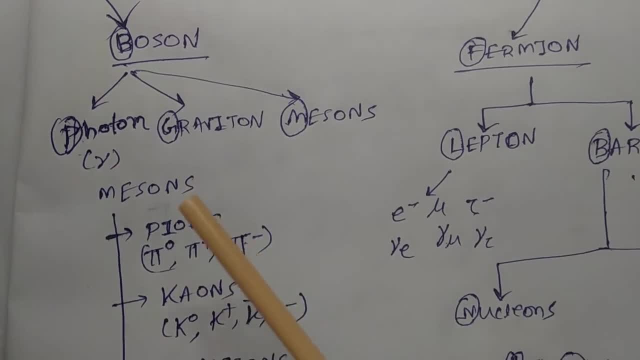 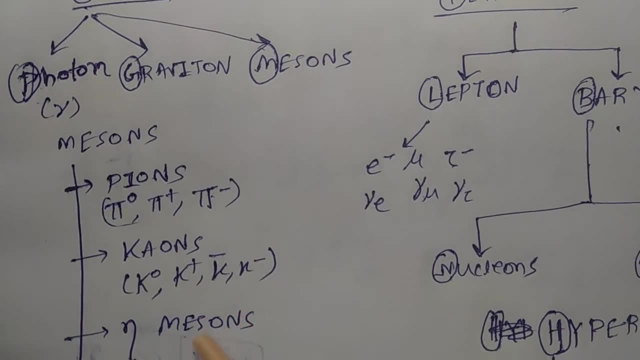 types of classification of mesons. A mesons they are pions, kions and etamesons Plus pi, minus pi, zero kions k, zero k plus k minus k, bar etamesons For fermions there are. 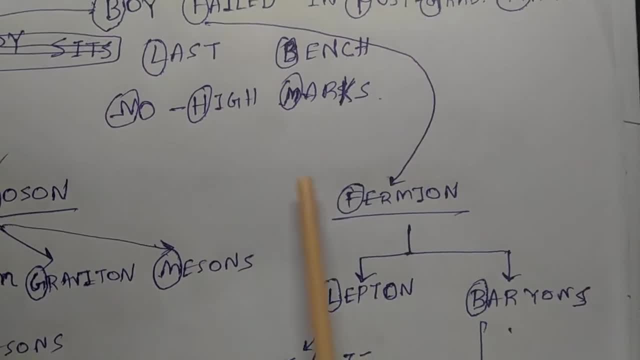 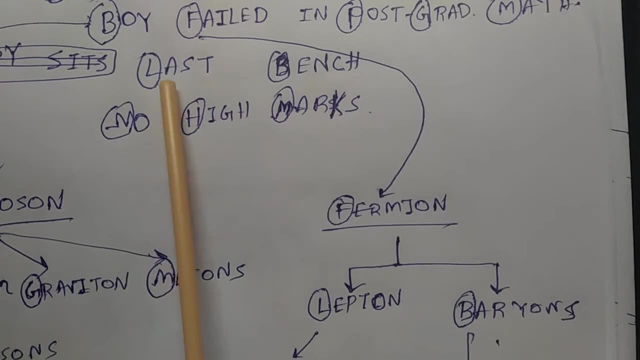 two types of classification: leptons and baryons. How to memorize them? You have to memorize the line last bench. The boy used to sit the last bench. Okay, L, L for leptons, B, B for baryons. 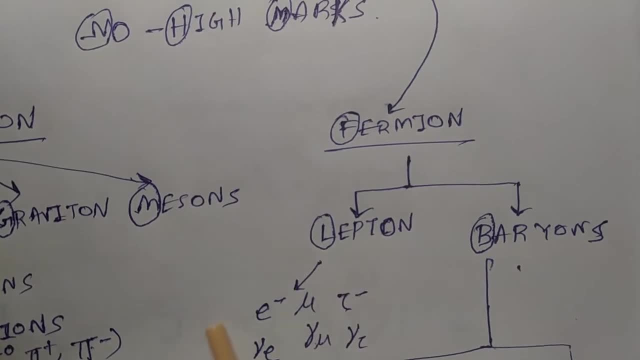 What are the classification of lepton? The classification: there are six types of classification of leptons. They are electron e neutrino, muon, mu, neutrino, tau, tau, neutrino. And the classification of lepton: there are six types of classification of leptons. There are: 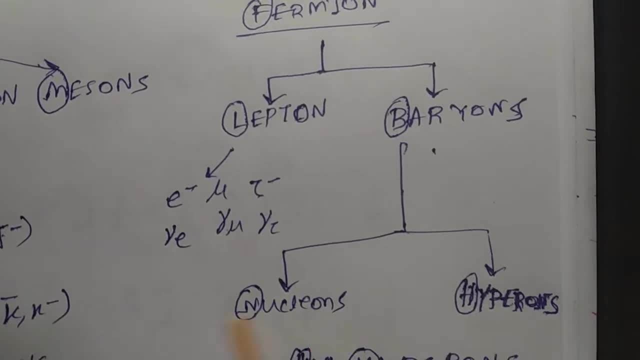 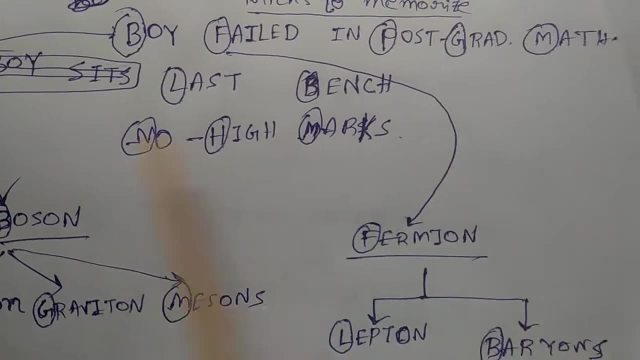 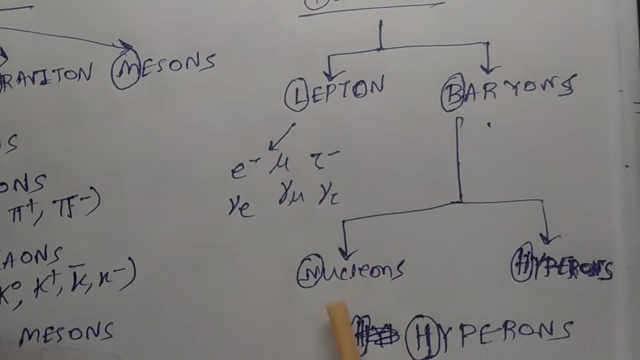 what is the classification of baryons? There are two types of classification of baryons: nucleons and hyperons. How to memorize them? The boy used to sit last bench. As usual, no high marks N, N for nucleons, H for high marks, H for hyperons. Nucleons, hyperons. You all know the classification. 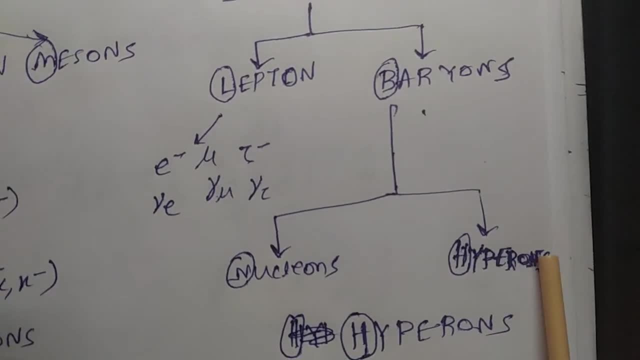 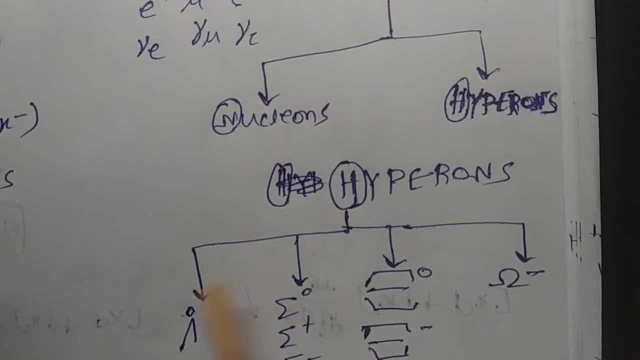 of nucleons. they are nucleon and proton. And what are the classification of hyperons, H hyperons? There are four types of classification of hyperons. They are lambda zero, sigma zero, lambda zero, sigma, cascade and omega. What are the classification of sigma, Sigma zero, sigma plus, sigma minus cascade? 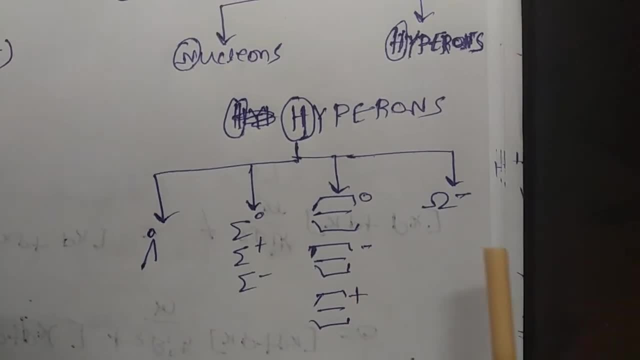 What are the classification of cascade, Cascade zero, cascade minus, cascade plus and omega hyperons? Thank you, These are the full list of elementary particles.